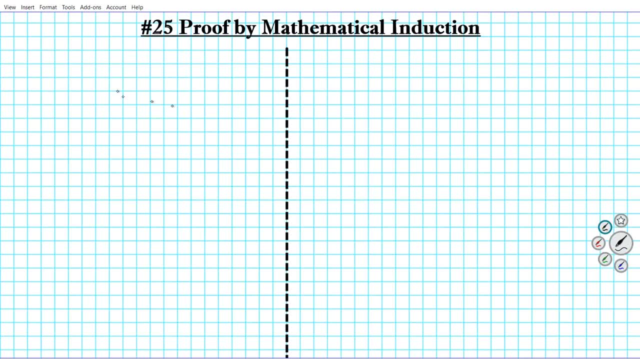 so we're going to prove. let's write down what we're proving. Problem 25, we're going to prove that 2 to the n is less than n, factorial for all integers, n Where n is greater than or equal to 4.. All right, so let's commence with the proof To 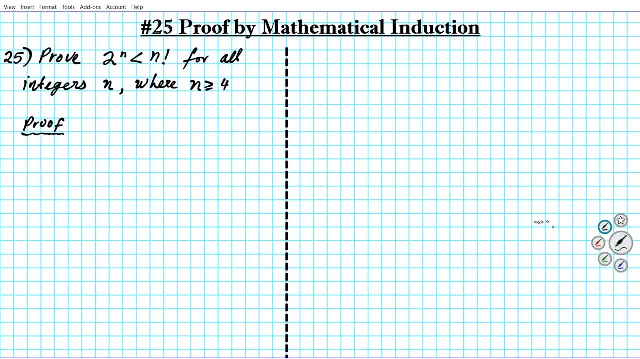 get us started, we're going to rewrite this inequality statement using SN. okay, So let's refer to the inequality statement 2 to the n is less than n factorial as SN S sub n. okay, So what we're going to do in? 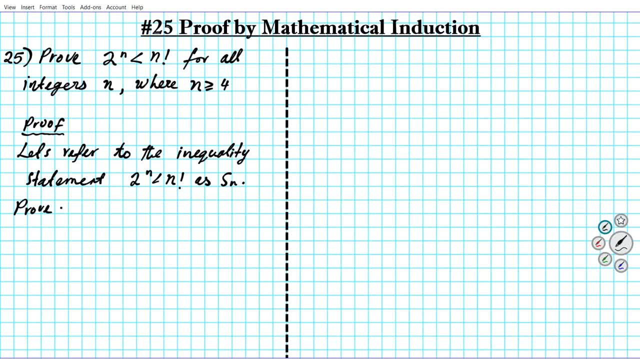 essence is we're just going to prove, we're trying to prove S sub n, which is that 2 to the n is less than n, factorial for all n And the set of natural numbers and n is greater than or equal to 4,. all right, This just means. 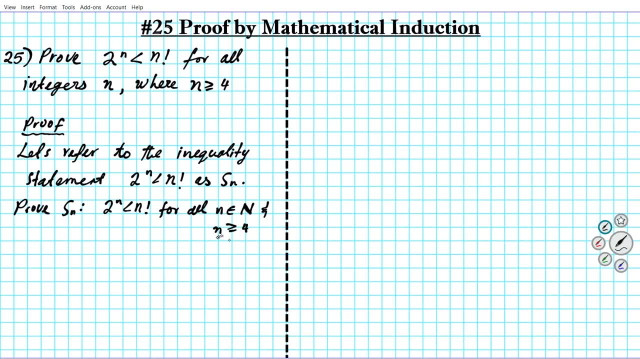 n is a positive integer and then n is greater than 4, all right, So let's go ahead and take a look at the procedure that we're going to use for this problem. So we're just going to be using the same standard procedure for proving math induction. 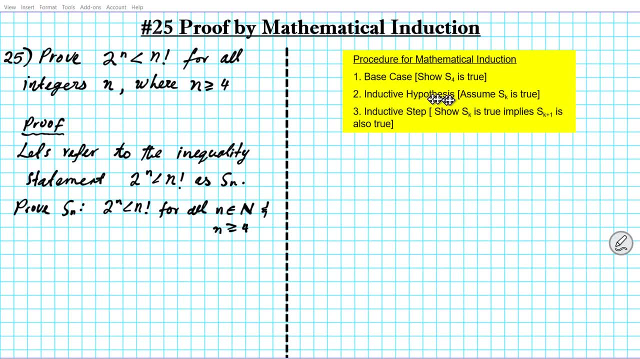 Which is you have a base case, which is the foundation, Inductive hypothesis and inductive step. If you can show that all the if you can show that the base case holds and then the inductive step holds, assuming that the inductive hypothesis is true, then it will hold for all. 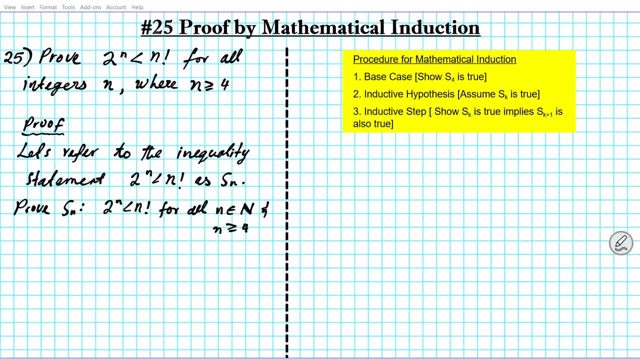 the conditions of your specified domain. all right. So something to keep in mind in this particular example is that we're starting with 4.. n is greater than or equal to 4. So we're going to first of all show that S4. 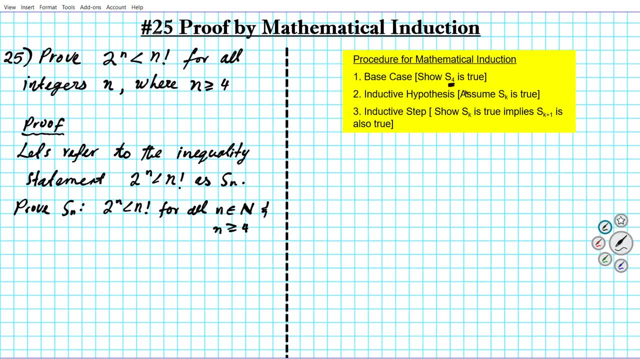 is true. A lot of math induction proofs starts at S1, so you need to be careful to pay close attention to the domain restrictions when proving by mathematical induction. okay, So we're going to show S1 as true first for the base case, inductive step: assume S sub. 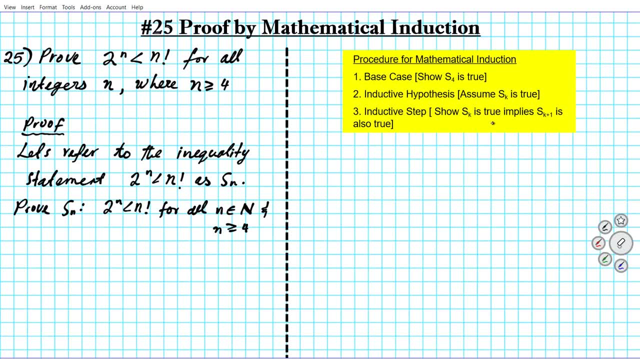 K is true. inductive hypothesis- sorry. and then we try to prove the inductive step, assuming the inductive hypothesis. If we can do that, then we know that that domino effect is going to take place for all integers in a specified domain. alrighty, 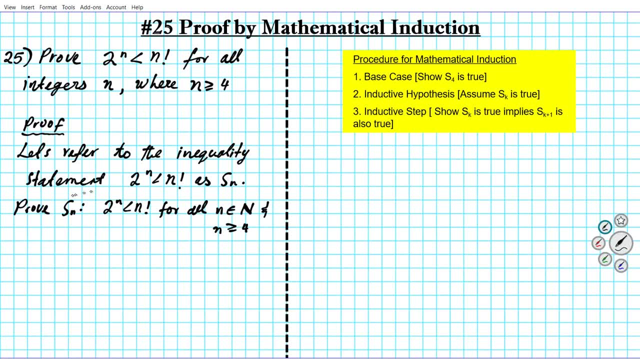 Okay, so let's do it. We are going to start with part 1, which is the base case. so what are we doing for the base case? So, for the base case, our task is to show that, enjoy um, show that S sub 4 is. 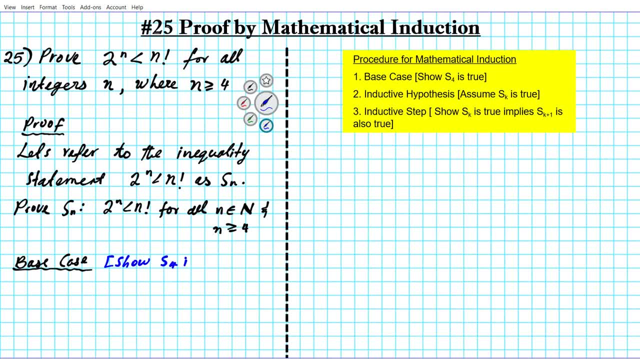 true. Okay, What does S sub 4 is true mean? If S sub 4 n is equal to 4, does this inequality hold? that's basically what we're trying to say. all right, so let's do it so. s of 4. 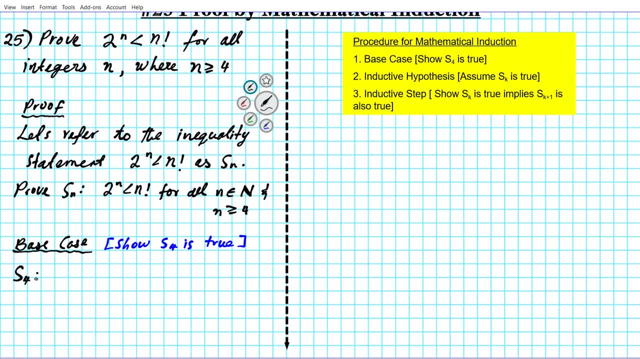 is what you get when you replace all the n's in the statement with 4. remember, s of n is 2 to the n- less than n- factorial. okay, so s of 4 is going to be 2 to the 4 is less than 4- factorial. we do not know if this is true, so we're going to put a question mark here. 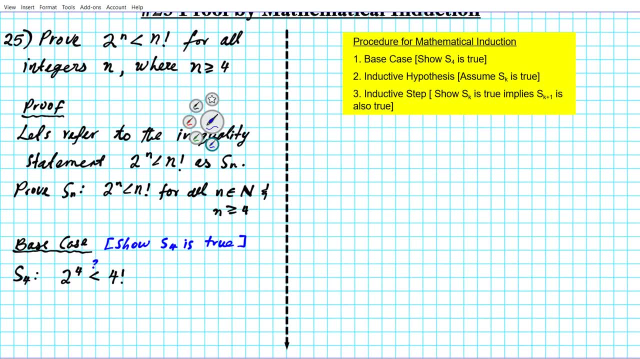 is, it is 2 to the 4, less than 4 factorial. so we're going to simplify both sides completely and then see if the inequality statement is true or false. so 2 to the 4 is 2 times 2 times 2 times. 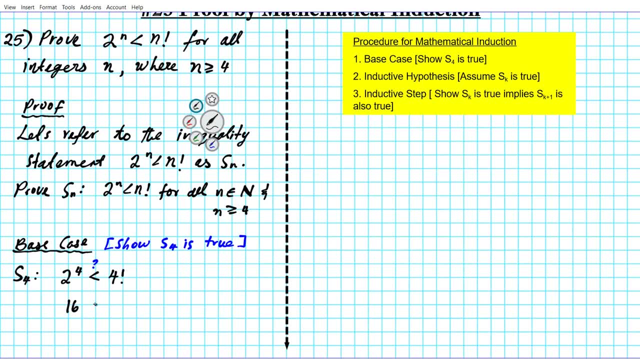 2 or 4 times 4, which is 16, is 16 less than 16. now remember what factorial is right. you count down all the way to 1 and you multiply the numbers in your in your countdown. so we're counting down from 4 all the way to 1 and we'll 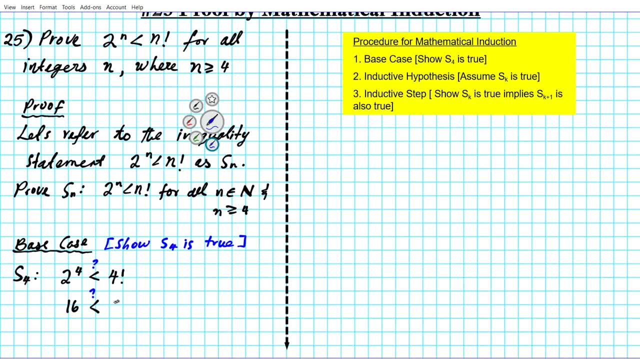 find a product of all those numbers in descending order. so we have 4. factorial is 4 times 3 times 2 times 1, bam like that. so it's 16 less than this number right here. well, let's see, it's 16 less than this number right here. so we're going to put a question mark here. 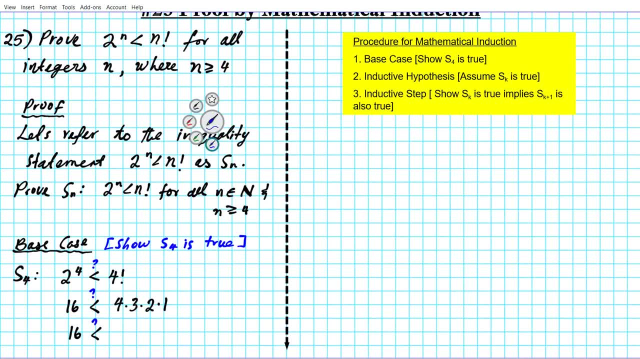 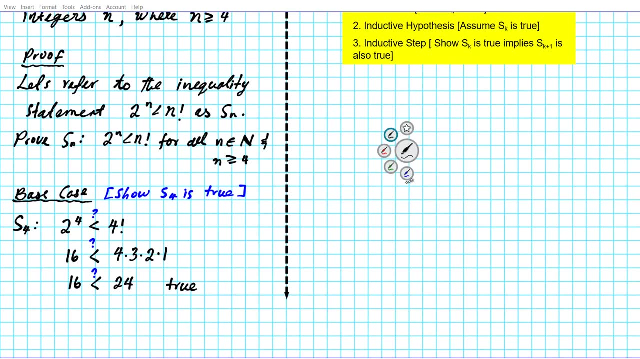 16 less than uh. 4 times 3 is 12. 12 times 2 is 24, is 16 less than 24. yes, it's true. so our base case, our foundation um, holds, so let's write that down. uh, the base case, the base case s of 4 is true. 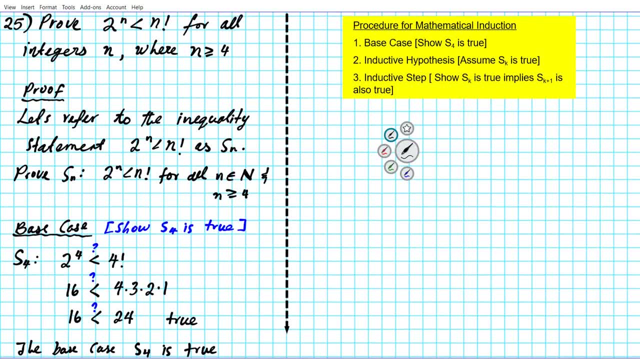 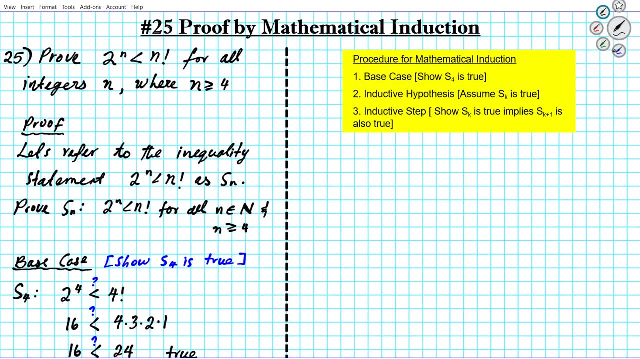 so we're done with part one of the proof. excellent, so we're now going to move on to our inductive hypothesis, which would be um what we use as the basis for the inductive step. okay, so part one: check. part two: inductive hypothesis. we're going to make an assumption here, okay. 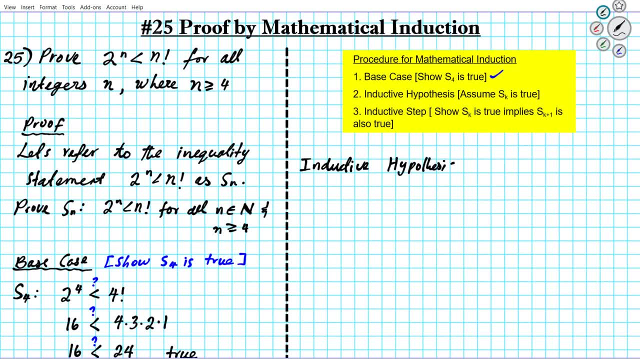 so your inductive hypothesis is: we're going to assume. we're going to assume that s of k is true. okay, s of k is true for some k in the set of natural numbers and k is greater than or equal to 4. all right, so let's go ahead and write down the formal statement. so, in the inductive hypothesis, 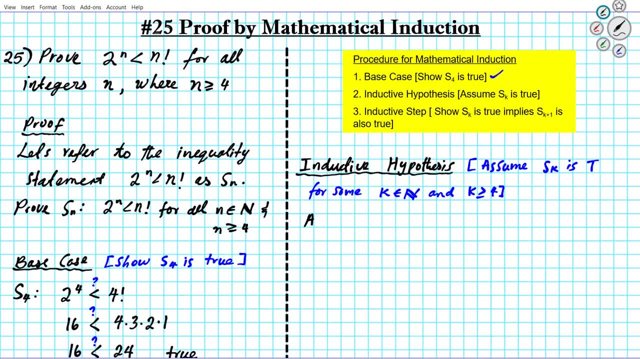 this is what we're going to do. we're going to assume that the statement s of k, which is 2 to the k, as less than k. factorial, you notice, s of k basically means that we replace all the ends with k. okay, because we're picking some arbitrary k in the in the 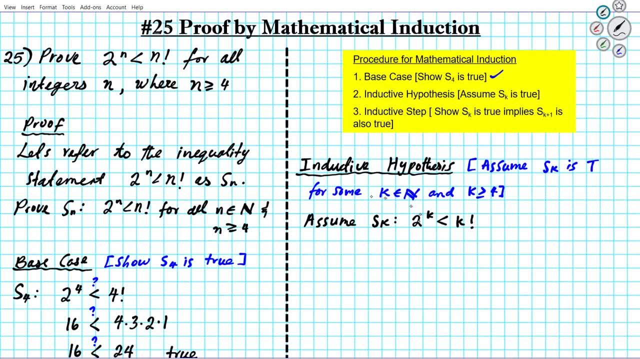 acceptable domain. all right. so for some random k and uh, the set of all integers where n is greater than or k is greater than or equal to 4, we assume that this is true. so assume that this statement is true for some integer k where, uh, first let's be. let's be specific here. 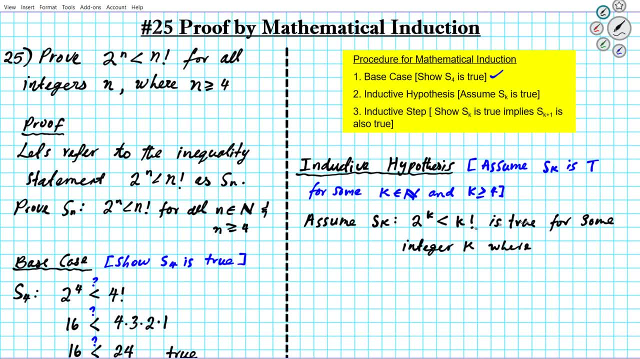 yeah, well, it's, it's suffice. we're basically looking at positive integers. for some integer k where k is greater than or equal to 4, when we put this constraint, k is, uh, greater than or equal to 4, it automatically means that k is positive. all right, so for some positive integer k, 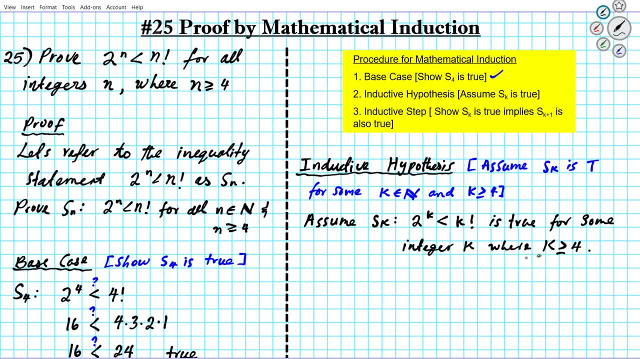 greater than or equal to 4. this is, this is sufficient, so let's assume that this statement is true. okay, so if we can now go to the next step, all right. so we make the assumption. now the next is the inductive step. inductive step. so what we're doing is basically setting up a domino effect to guarantee that if one sequence 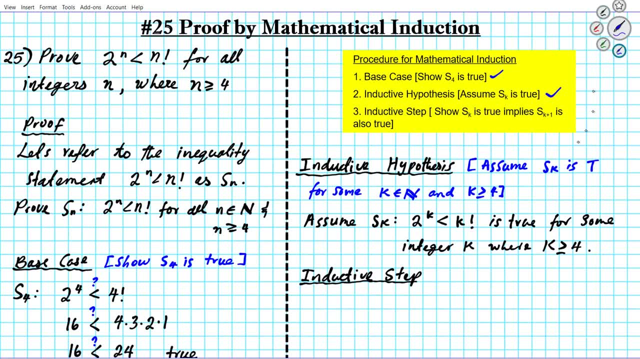 of steps works, then it has a domino effect on every other step for all the integers. all right, so we don't have to do it for every single case. if we can just use these inductive hypothesis and inductive step, then we can show that it will always hold true. 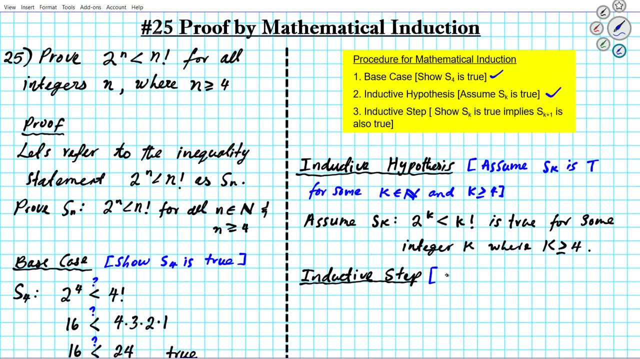 all right. so for inductive step. our task here is to show that S sub K is true. follows that the next step: S sub K plus one is also true. All right, So we're going to start with S sub K plus 1 and see if we can use this inductive hypothesis. 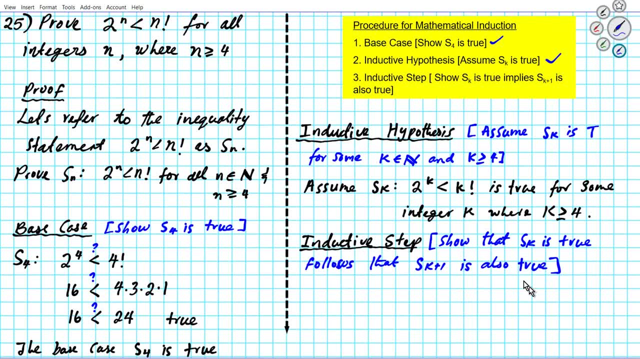 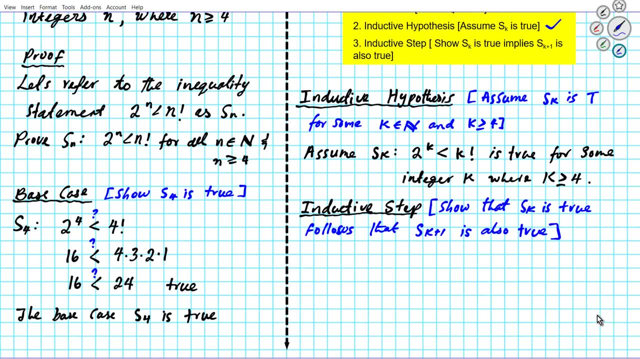 to show that S sub K plus 1 is also true based on our inductive hypothesis. All righty, Okay, so let's start with S sub K plus 1.. So S sub K plus 1, the next step. What is the S sub K plus 1?? 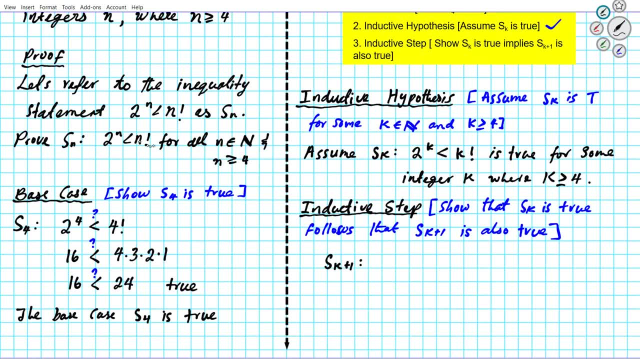 We just substitute K plus 1 for the ends, right. So we have 2 to the K plus 1.. Now can we show that this 2 to the K plus 1 is less than K plus 1 factorial. That's the goal, okay. 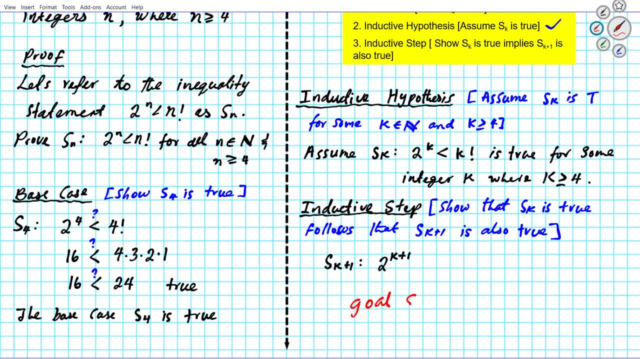 So let me just put a side note here. So goal is to show. goal is to show that 2 to the K plus 1 is less than K plus 1.. Using: we have to use the inductive hypothesis, using S sub K. 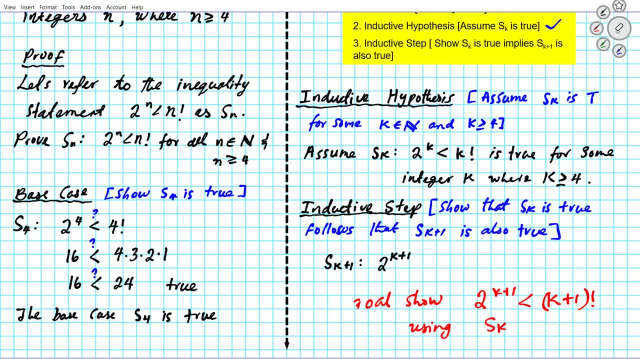 So that's what we're going to do, okay, All right, so we have the left side down. we want to show that it's less than K plus 1. All right, so first thing we're going to do is apply the property of exponents. 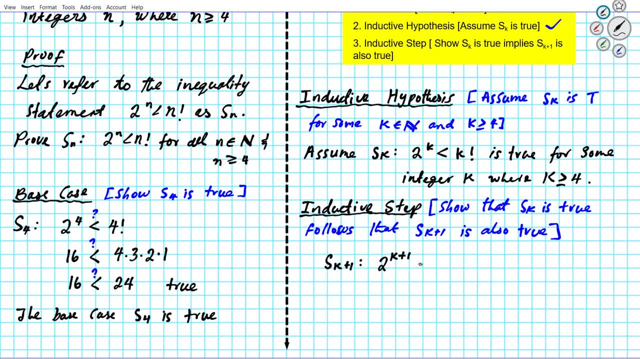 When you multiply two exponents of the same base, you add the power. So we're going to go backwards on that. All right, So we have the sum of power. so it's basically the product of two exponents of the same base. 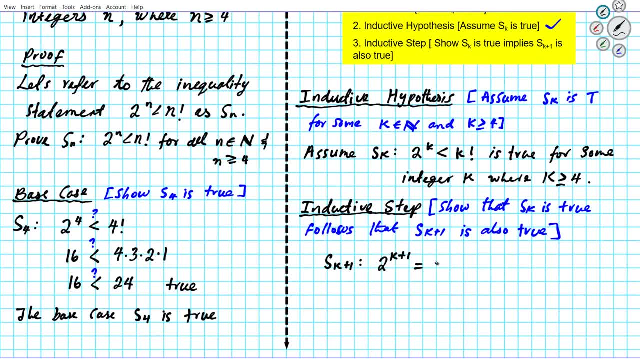 and the exponents will be the addends of your power. So 2 to the K plus 1 is 2 to the K times 2 to the first power. Bam, All right, So the goal here is when you break it apart. we want to see. can we make any substitutions? 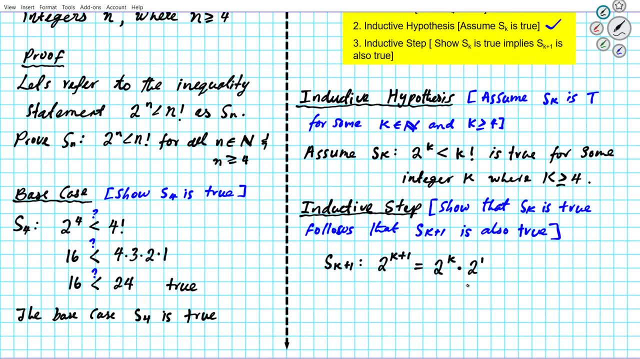 here utilizing our inductive hypothesis. Now you notice we have a 2 to the K inductive In our inductive hypothesis. But what do we know about 2 to the K? We know that it's less than K factorial. okay, 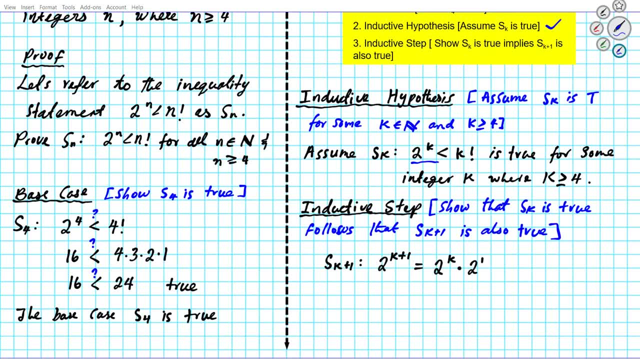 So let's make a substitution here. So, since 2 to the K is less than K factorial, that automatically follows that this statement right here- 2 to the K times 2, is going to be less than what. It's going to be less than K factorial times 2.. 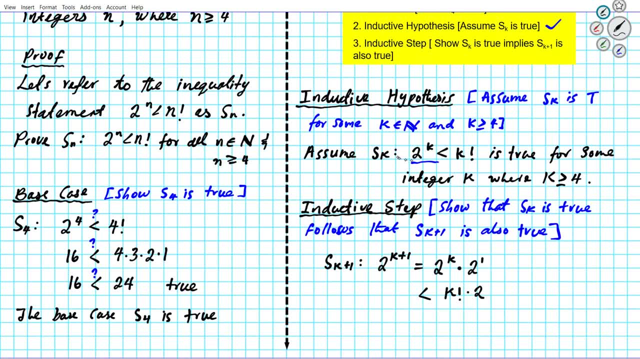 Okay, Using our inductive hypothesis, all right, Since 2 to the K is less than K factorial, okay, So check this out. If you have, 2 to the K is less than K factorial from our inductive hypothesis and you multiply, 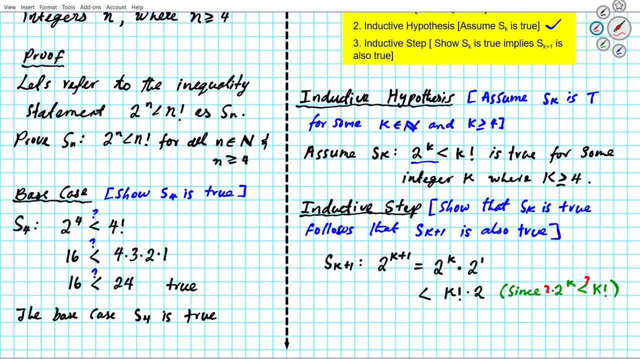 both sides by 2.. Bam, bam. What do you have? You have a situation where 2 times 2 to the K is less than K factorial times 2, right? So that's what we're doing, Since 2 to the K is 2 to the K, times 2 is less than K factorial times 2, and 2 to the 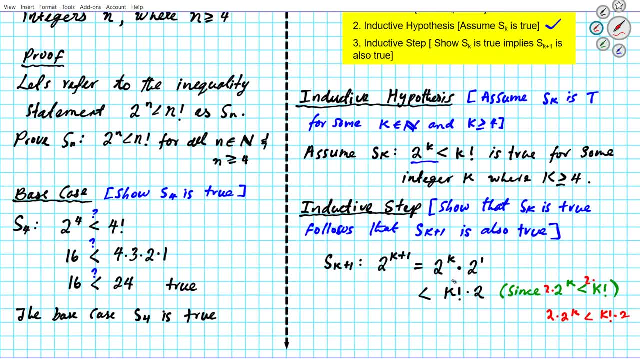 K plus 1 is equal to 2 to the K times 2, then we can just make a substitution: We know for sure that 2 to the K plus 1 is less than 2.. Okay, We know for sure that 2 to the K is less than K factorial times 2, because these two 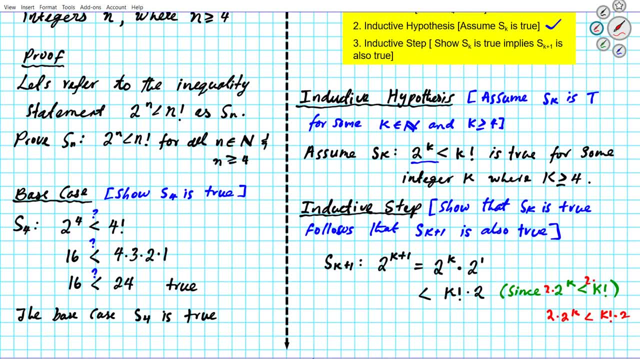 are exactly the same. Okay, All right, Bam, So we have that right there. Make the substitution. Okay. So now what do we know about K factorial times 2?? Okay, So just remember that this we have right here is based on the assumption that we made earlier. 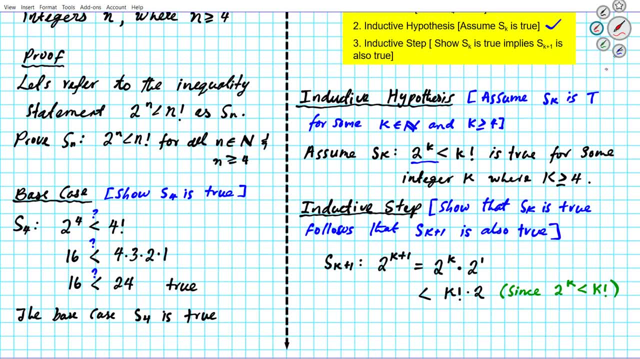 over here. Okay, So we have K factorial times 2.. We're going to take a look at the domain of our proof and see how we can use that to see how this compares with K plus 1 factorial. Okay, So what do we know about the domain? 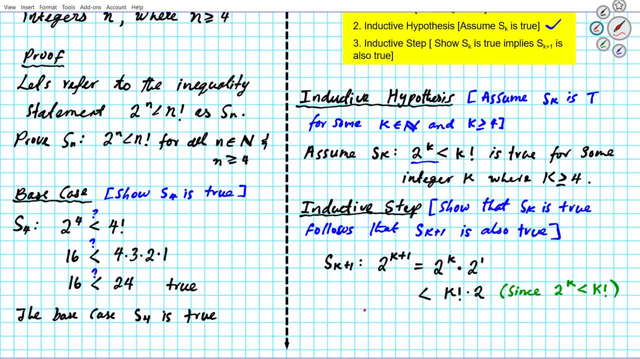 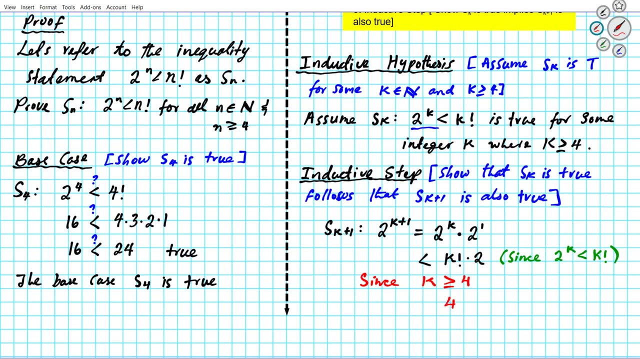 We know that K has to be bigger than or equal to 4.. All right, So since K is greater than or equal to 4, how does 2 compare with K? Okay, If K is greater than or equal to 4, that means 4 is less than or equal to K, And we know for. 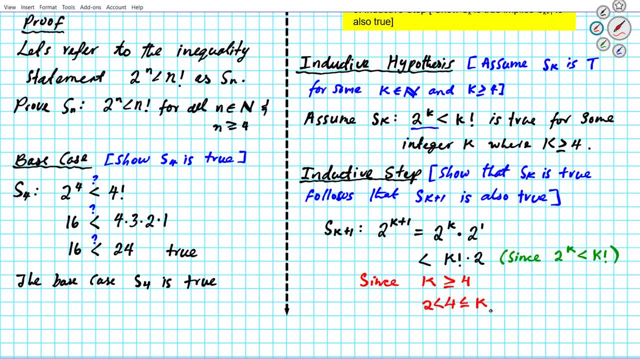 sure that 2 has to be less than K, because 4 is greater than 2.. Okay, So since 2 is less than 4 and 4 is less than or equal to K, it follows that 2 is less than K. 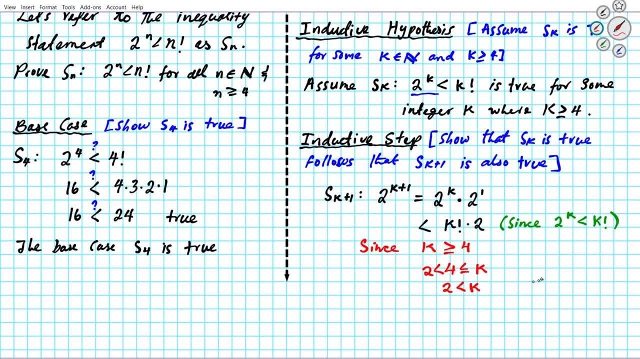 All right, Now how does K compare? how does 2, sorry- compare with K plus 1?? If 2 is less than K, then for a certainty 2 has to be greater than or equal to K. All right, 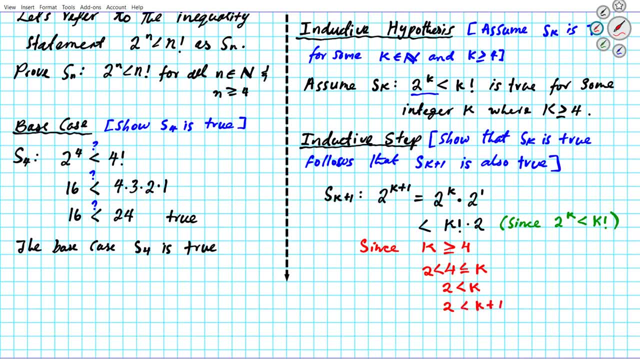 So 2 has to be less than K plus 1, because K is a set of integers that are greater than 4.. All right, Now let's go ahead and see what happens. what if we multiply both sides of this inequality by K factorial? 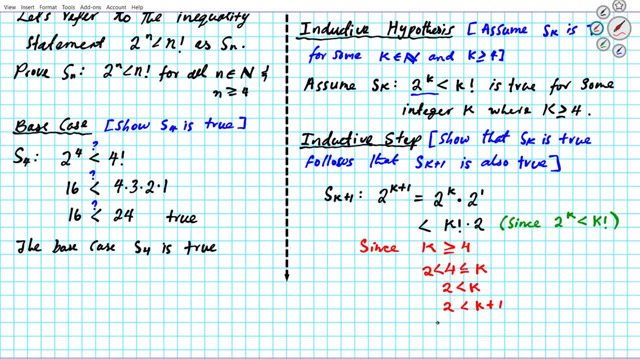 All right. So if we multiply both sides by K factorial, we know that 2, I mean K factorial, K factorial times 2.. It's going to be less than K factorial times K plus 1.. How do we know this? 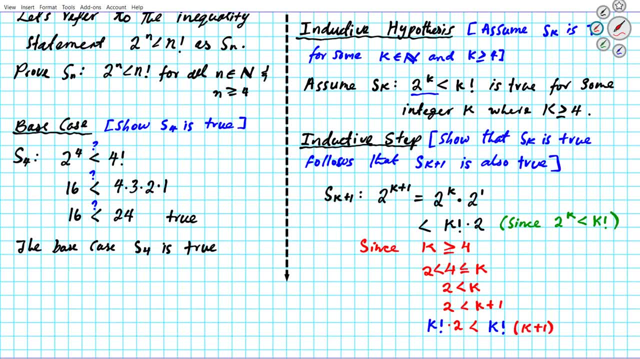 How do we know this? Well, K, factorial, by definition, is always greater than 0.. All right, If you multiply an inequality with the same positive number both sides, the orientation doesn't change. Okay, The magnitude doesn't change, All right. 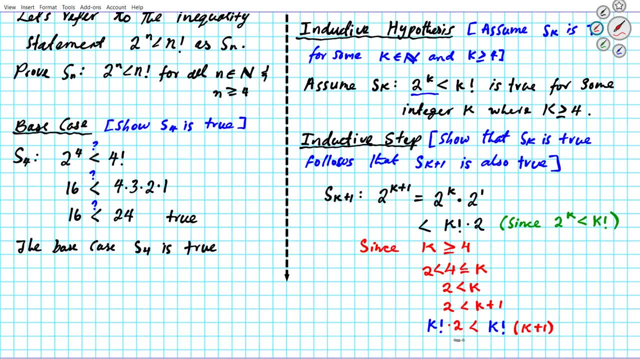 So if you multiply by negative, then that's when the inequality flips, Since K factorial is bigger than 0, when you multiply an inequality by that, the inequality does not change, All right, Since K factorial is greater than 0, by definition the factorial starts from 1.. 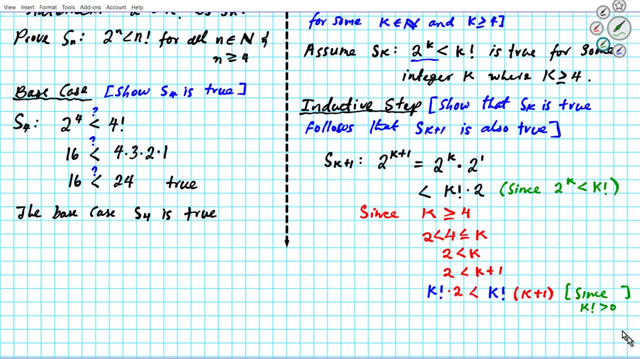 Okay, All right. So now we have this scenario right here. What we can do is make another substitution. Okay, So look at what we had earlier. We said 2 to the K plus 1 is less than K factorial plus 2.. 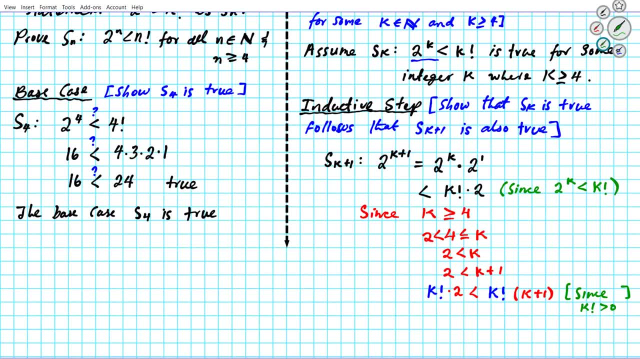 And now we have another situation: The same K factorial times 2, how does it compare to what we just created? It's less than K factorial times K plus 1.. All right, So, since K factorial times 2 is greater than 2, to the K plus 1, and K factorial times 2. 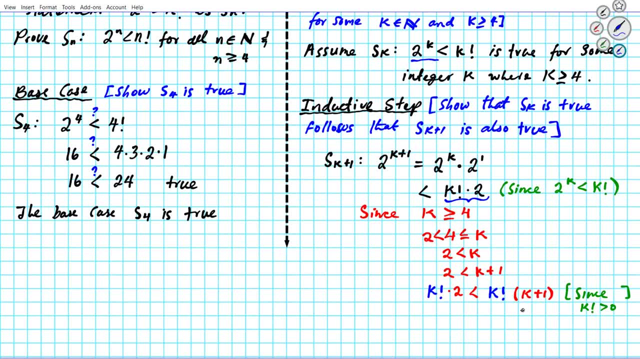 is less than K factorial times K plus 1, if we use the transitive property of inequality, what can we say? You know what? Let me just write this here so it's easy for you to see what's going on. All right, 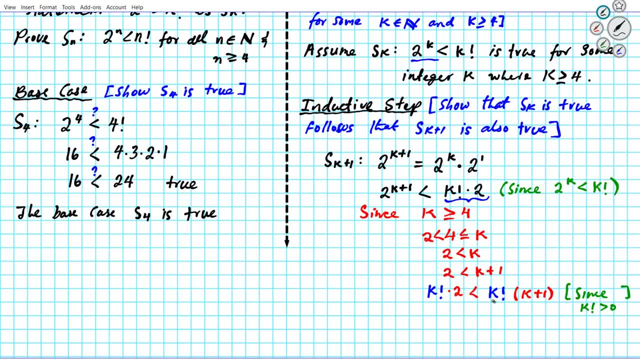 So 2 to the K plus 1 is less than this, and this is less than that. Using the transitive property of inequality, it follows this: All right, Inequality. it follows that, which follows that 2 to the K plus 1 is what. 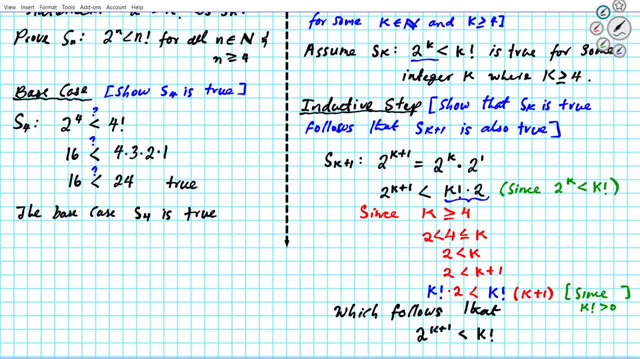 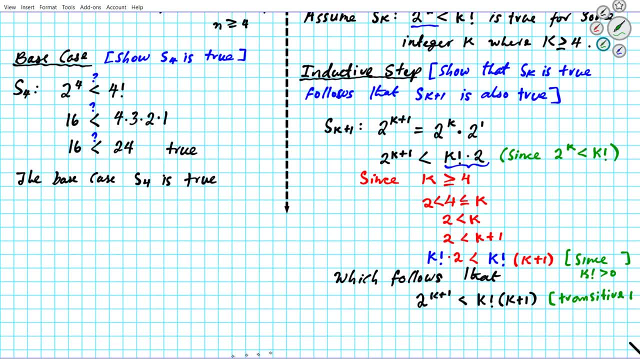 Okay, I'm going to write it down here: Transitive property of inequality. Hopefully you remember that Transitive property of inequality. What on earth is the transitive property of inequality? Let's take a look at that real quick. So the transitive property of inequality just states that if A is less than B, all right. 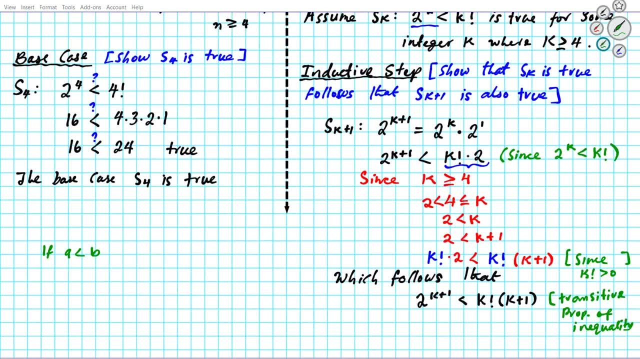 A is less than B, All right, All right. So if A is less than B and B is less than C, then what Then? A is less than C. It's pretty much. it's pretty intuitive. Okay, All right. 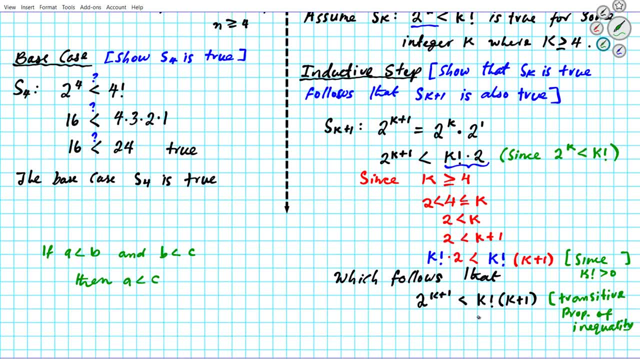 So that's what we're using here is the transitive property of inequality. Now we're going to use the definition of factorial to combine, to simplify the right side. All right, What is K factorial times K plus 1? K factorial times K plus 1 is like we are reassembling the factorial numbers. 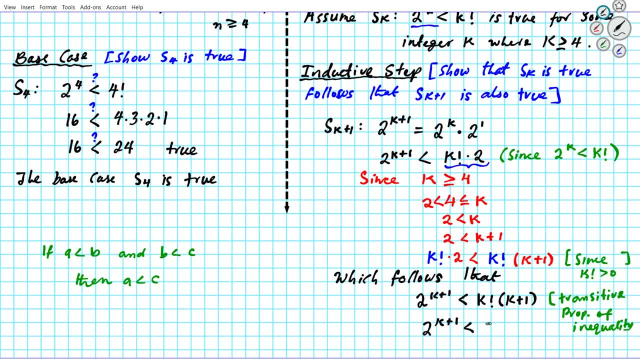 Okay, K factorial times. K plus 1 is simply K plus 1 factorial. All right, Just like. for example, if you have 5 factorial, is this equal to 4, is equal to what is 5 factorial. 5 factorial is 5 times 4 times 3 times 2 times 1.. 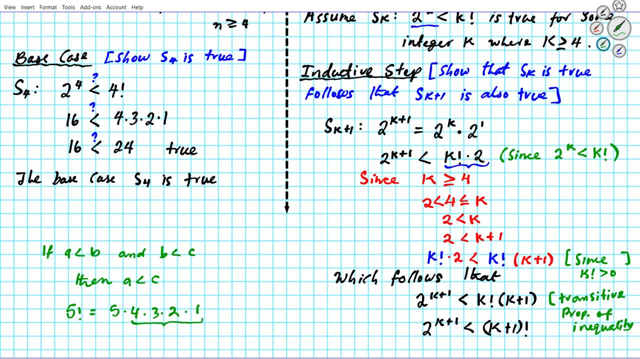 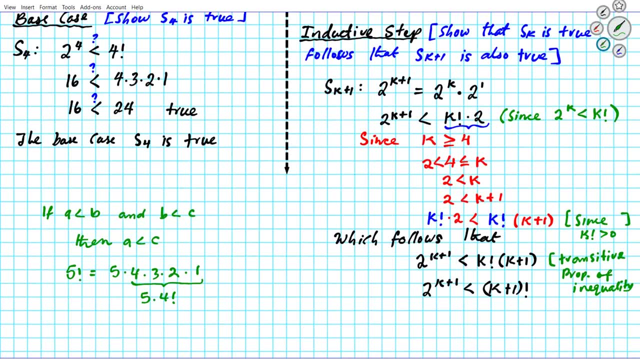 All right, You assemble these four digits together, that's 4 factorial, isn't it? So 5 factorial is the same thing as 5 times 4 factorial. All right, It holds for all N's right. So N factorial is the same thing as N times N minus 1 factorial. 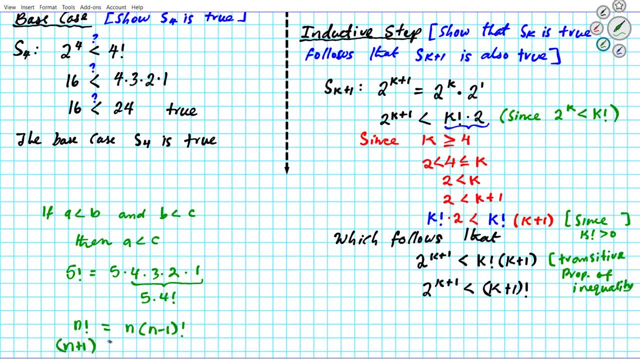 If you do N plus 1 factorial, which is what we're doing right here, is the same thing as that number, N plus 1, times the number before it: factorial, N, factorial. Okay, In this problem, in this proof, we're going backwards. 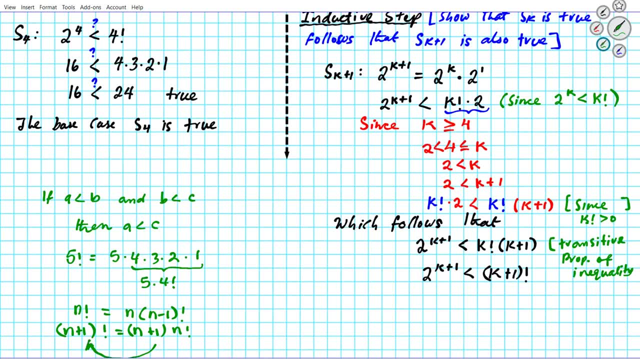 We're assembling the numbers, Okay, So the number before K plus 1 is K, so K factorial times K plus 1 is simply K plus 1 factorial Voila. This is exactly what we're trying to show, All right. 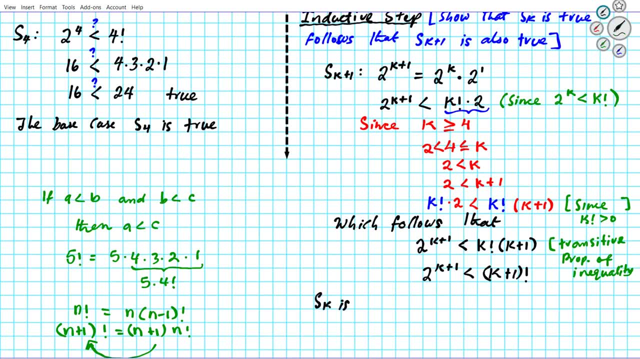 So we've been able to show that S sub K is true. Follows that. Follows that S sub K plus 1 is also true. That is also true, All right, So let's go ahead and write down our conclusion. 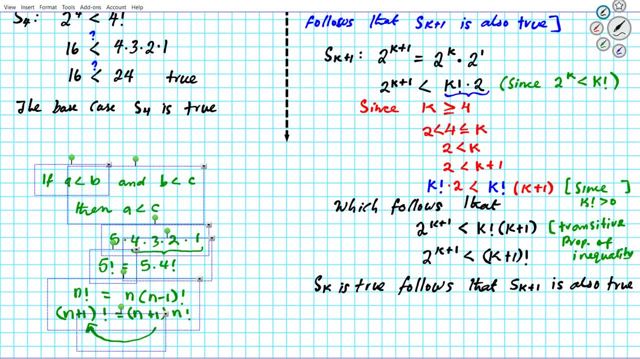 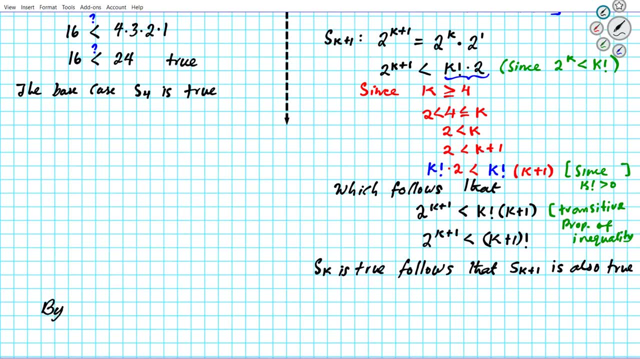 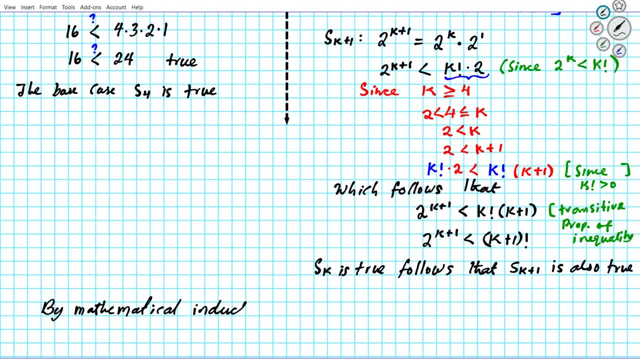 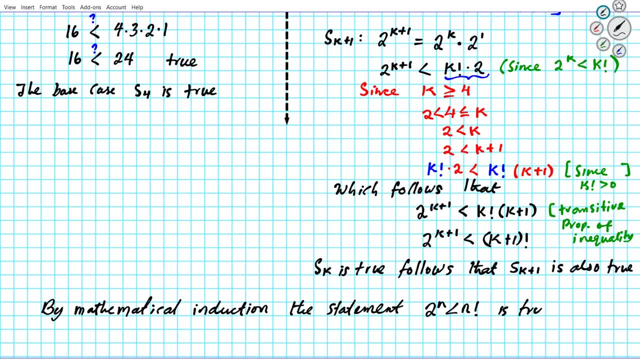 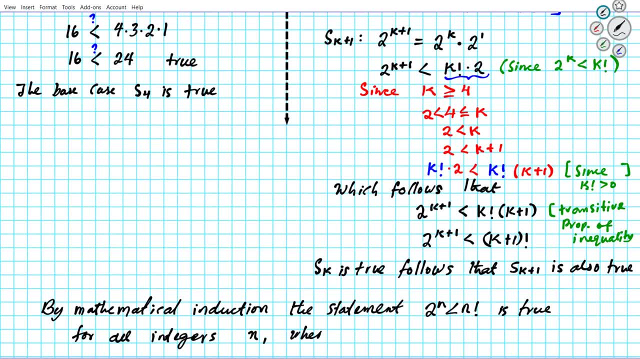 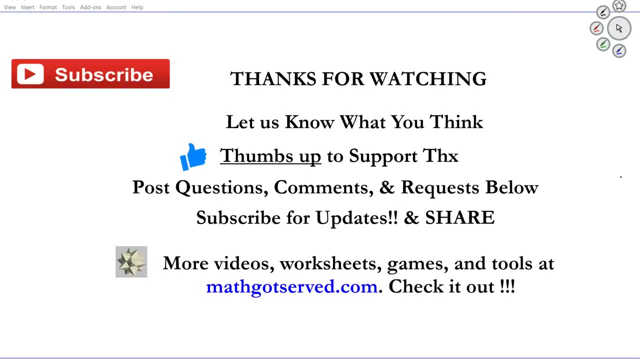 By mathematical induction. By mathematical induction where n is greater than or equal to 4.. Alrighty, and I put you a nice little box of accomplishments to indicate that you've concluded the proof. Thanks so much for taking the time to watch this presentation. Please help support our 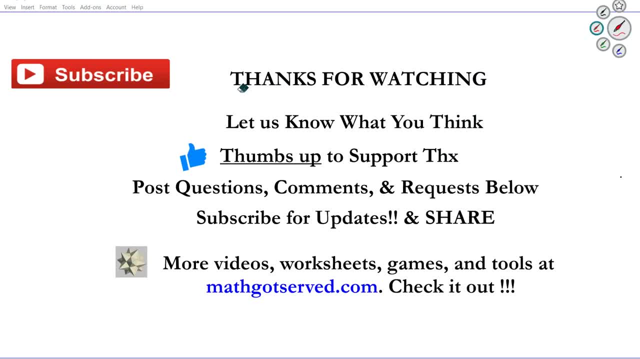 channel by liking, subscribing and sharing the contents of this presentation with your friends. Tons of support resources can be found on mathgotservedcom. Also, don't forget to take a look at the links in the description below to gain access to a wide collection of math induction proofs. 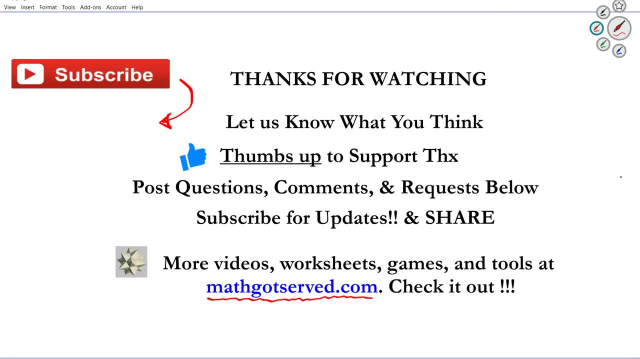 that we have also accessible at mathgotservedcom. Thanks again for watching and we'll see you in the next video. Bye, bye.